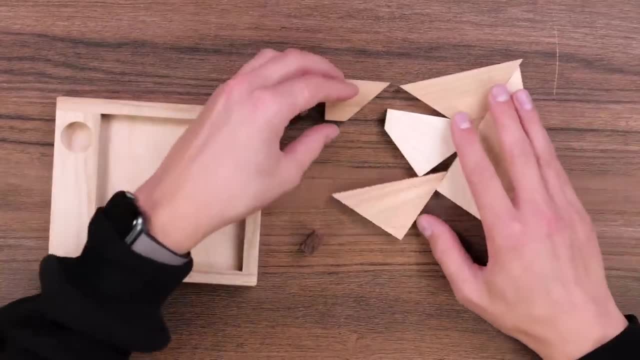 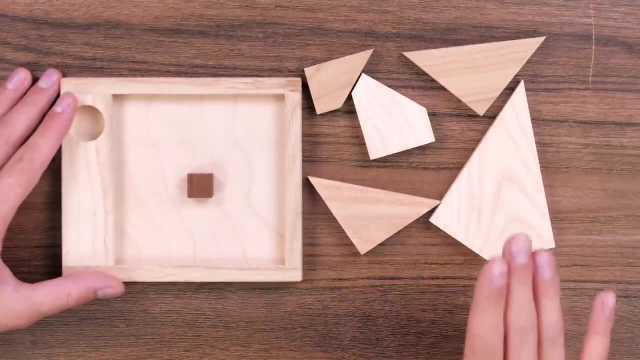 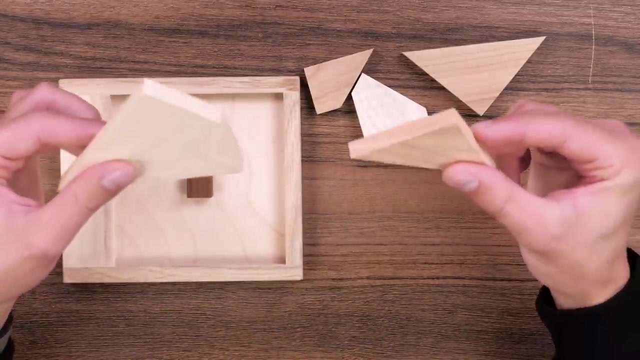 So here we have a black square And 1,, 2,, 3,, 4, 5.. Not very big or big. Quadrangles, pentagons, polygons and triangles of different shapes. We can put these pentagons and polygons. 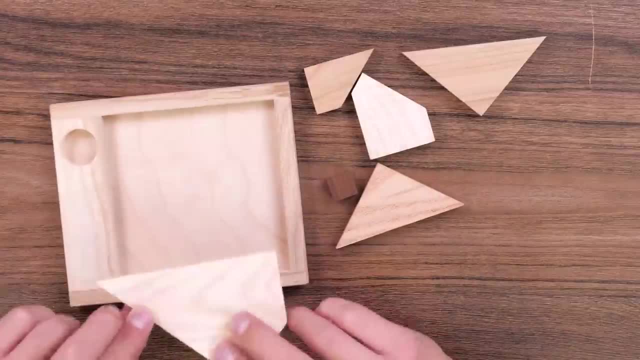 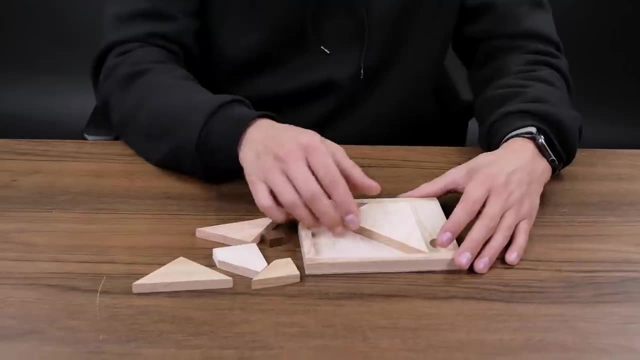 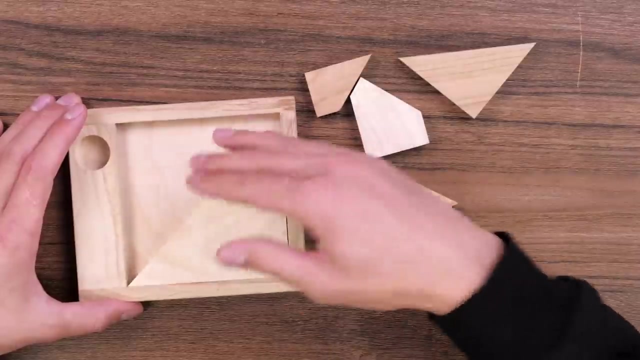 inside this frame. You can turn it over or not, but the most important thing is to do it in a horizontal position, not vertically. You are able to do it anywhere inside the frame. You can put it as you wish, like this, this way, As I understand the biggest element. 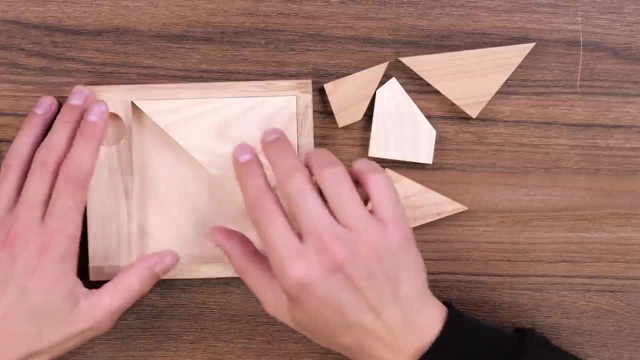 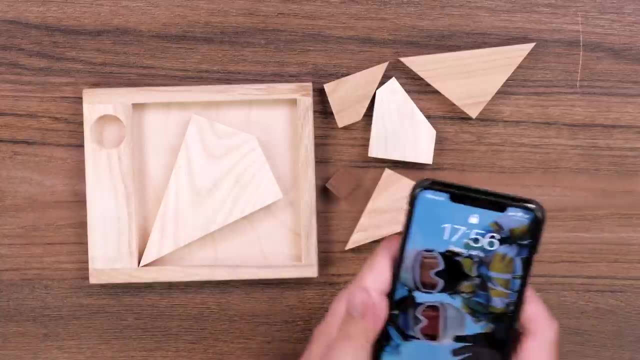 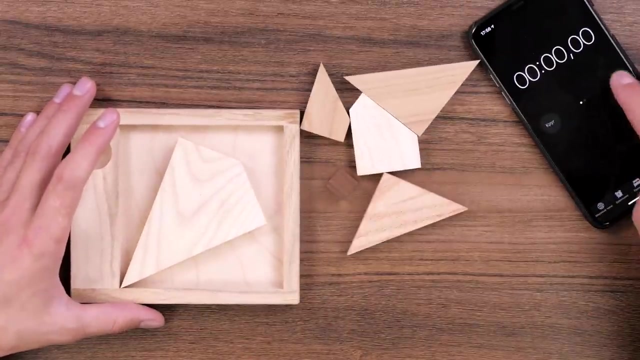 will lie close near the wall, But I'm not sure. I know that many puzzles have different interesting solutions. By the way, I forgot to time it. Let's try to speed-solve the puzzle, as we usually do, as quickly as possible, if it works out. So let's try to do something. 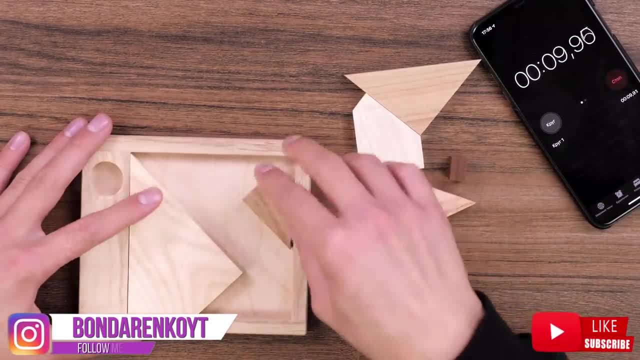 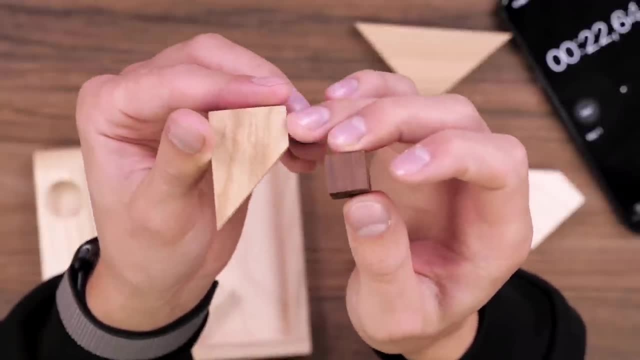 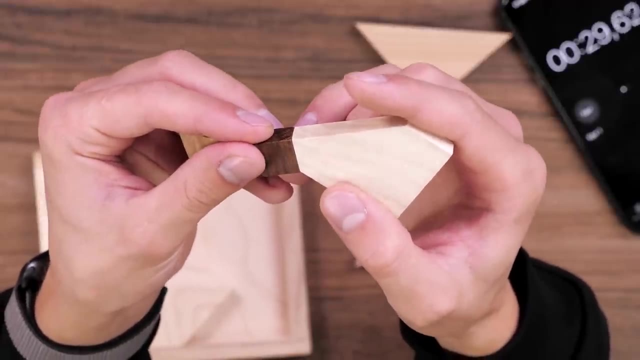 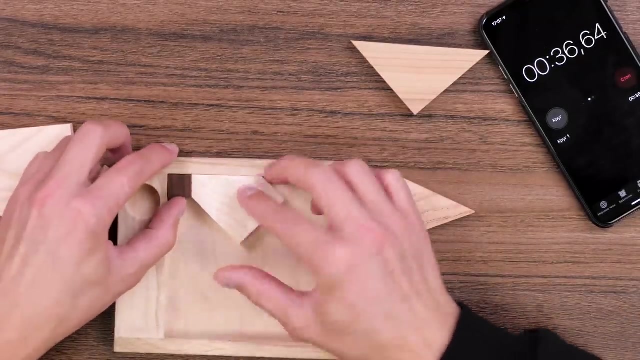 Uh-huh, It's lying really tightly. I noticed that this side of the black square is equal to the side of this stripe, And we also have some more elements with equal sides. Hmm, Interesting. Let's try to solve it this way. Okay, look at this. Already not bad. 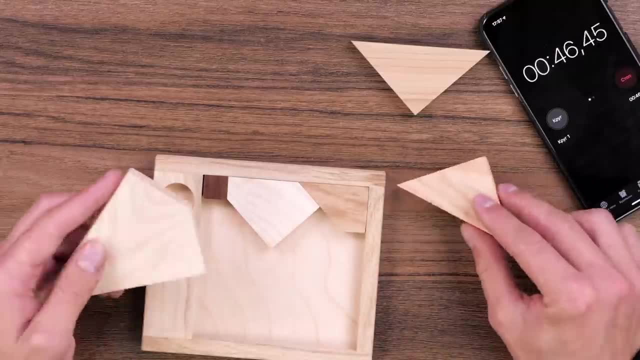 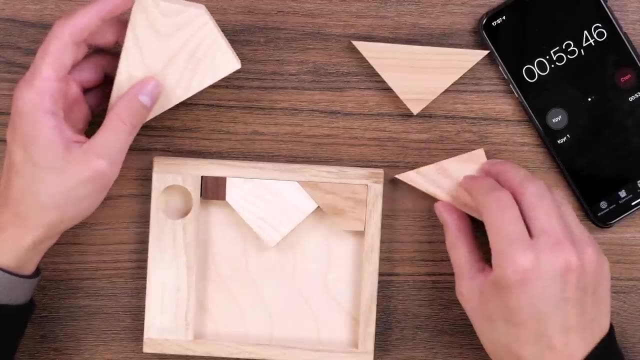 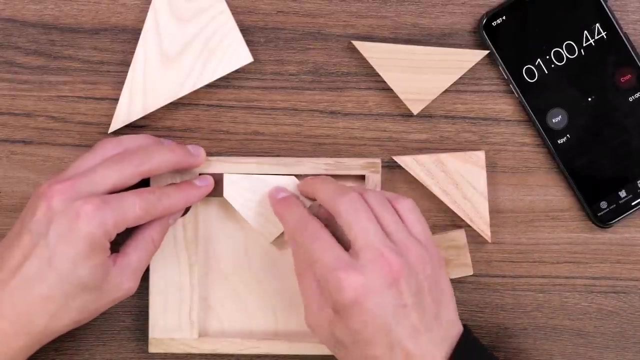 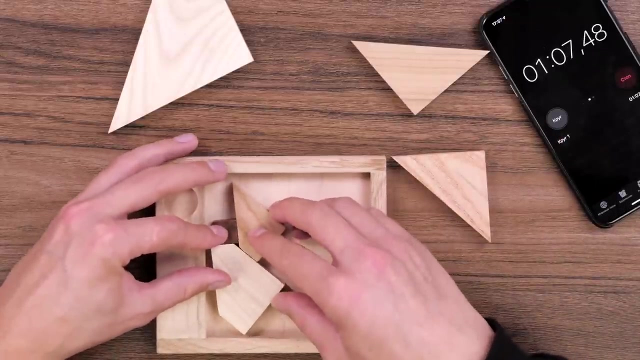 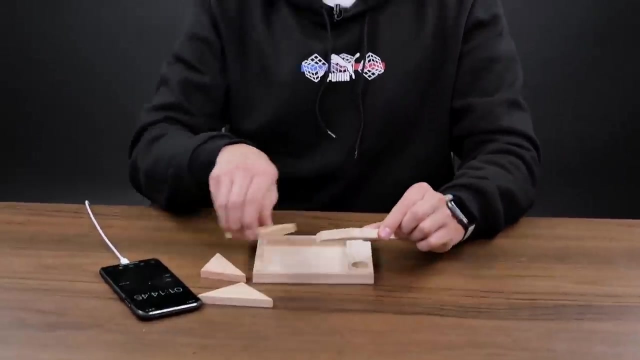 It looks good. We have to come up with these parts, But it won't work out Because of the triangle that will be left here. Okay, We will do it, Let's try another side. So it's not so easy. We will start from the biggest part, Because 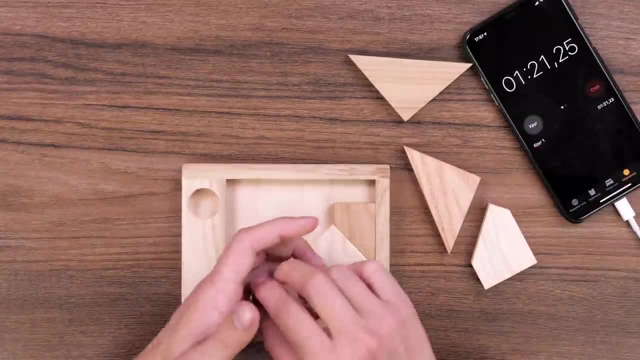 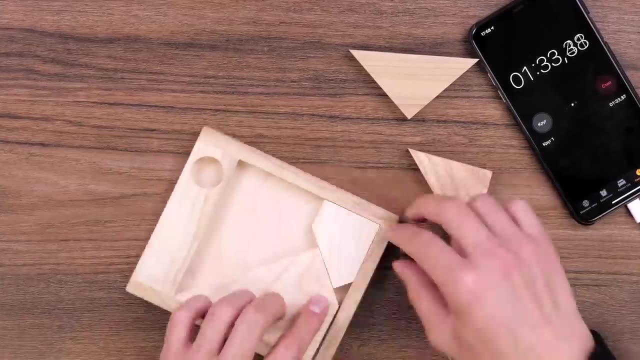 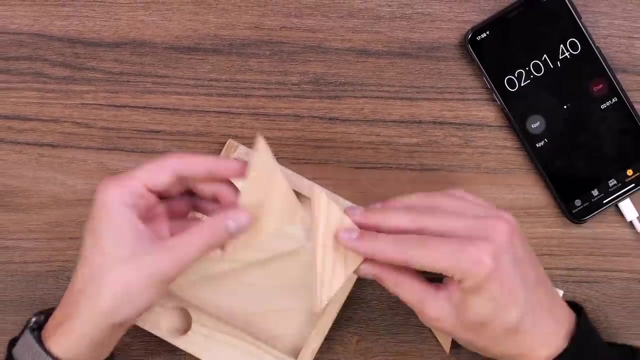 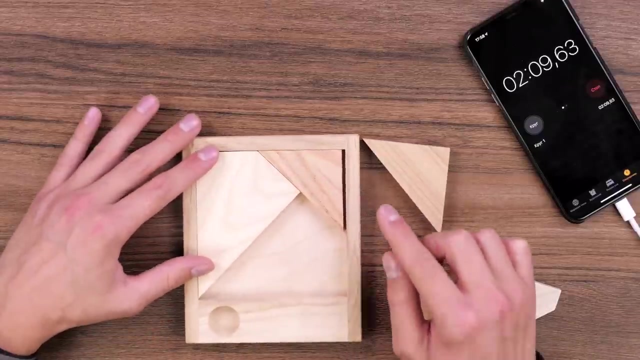 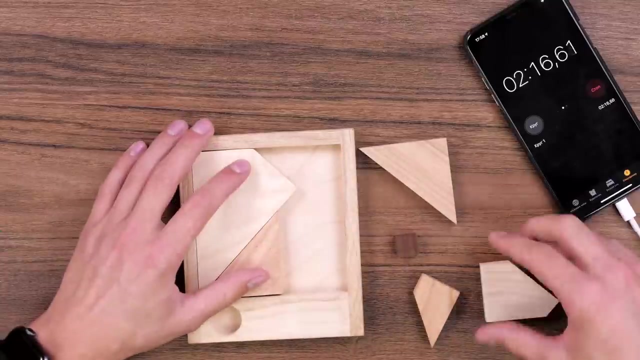 I don't see the other variants Here. Uh-huh, Here It is not hard to see that there is a free space if we put the detail wrong, Because we need to use properly each square millimeter of this puzzle. Maybe that way I will be close. 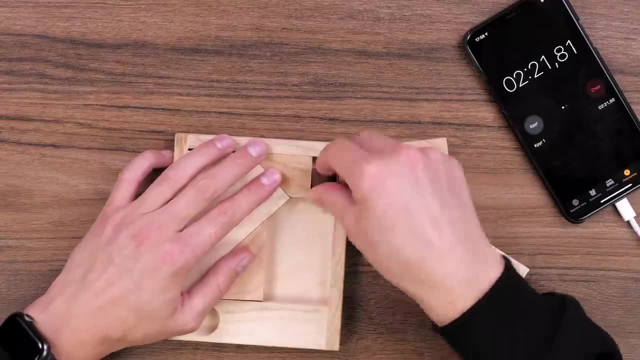 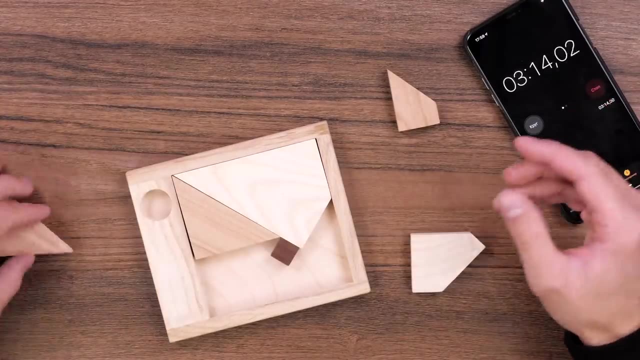 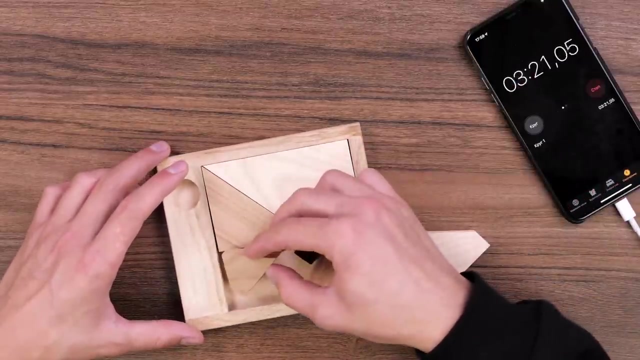 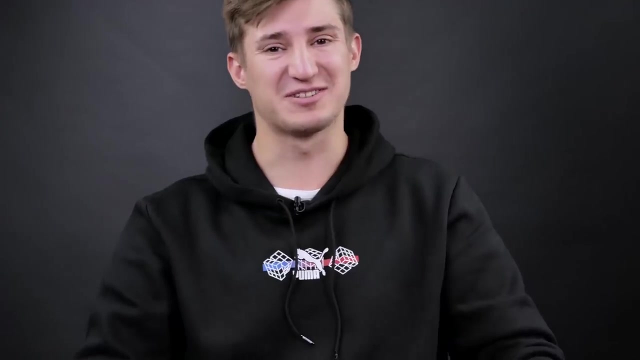 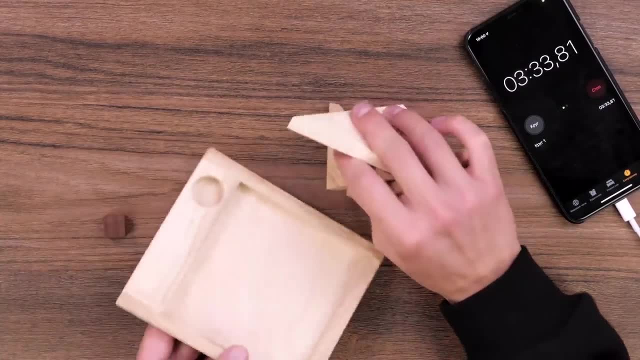 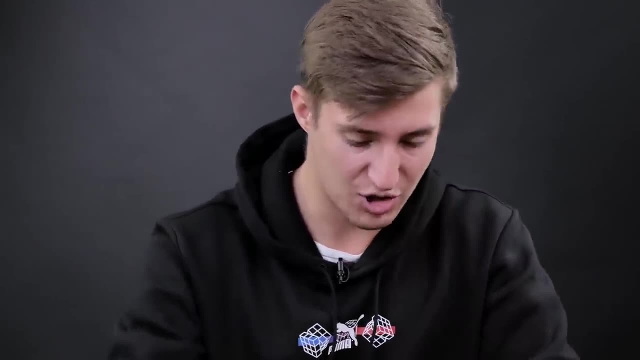 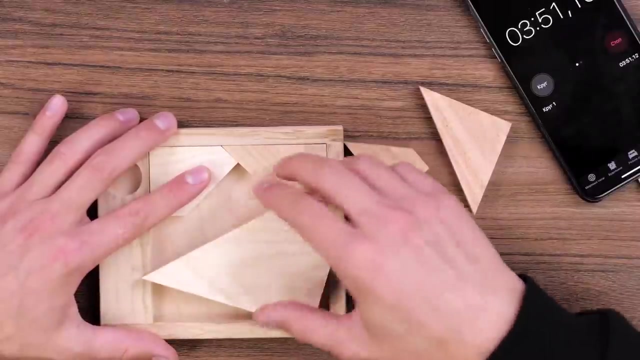 Okay, Let's try once more. There are a lot of puzzles like this. There are a big variety of pieces, cuts that you can put and not inside the frame, different pieces. Oh, look at this Right now. I have proved myself that this. 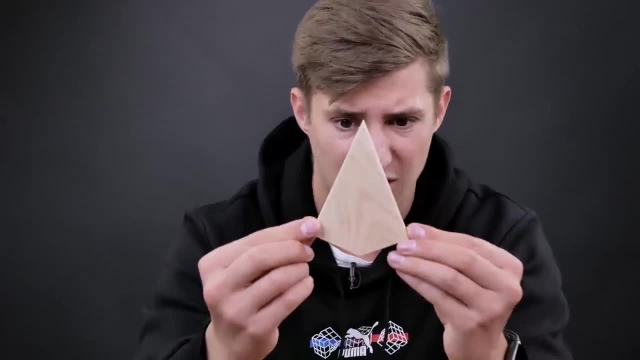 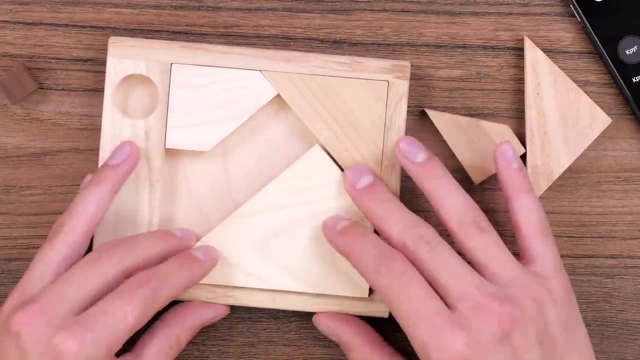 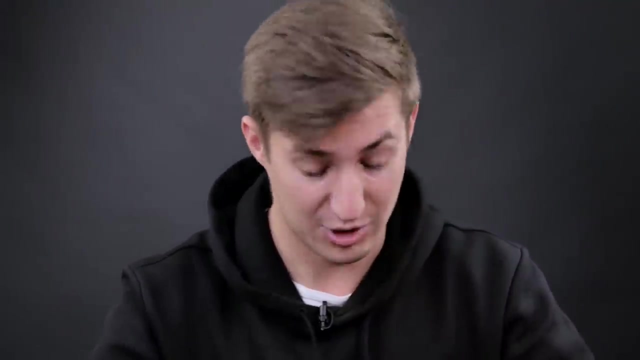 detail isn't totally symmetrical, Though it looks like a symmetrical arrowhead, But look, if I'll put it here it won't fit in, But if I turn it over it fits perfectly. That's what I expected. Well, what I was talking about, Oh, that we can turn the details over any way we want. 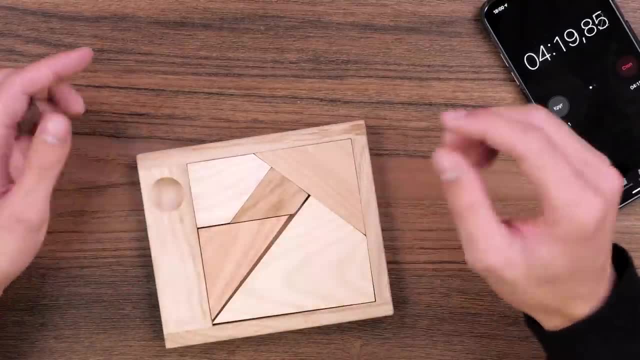 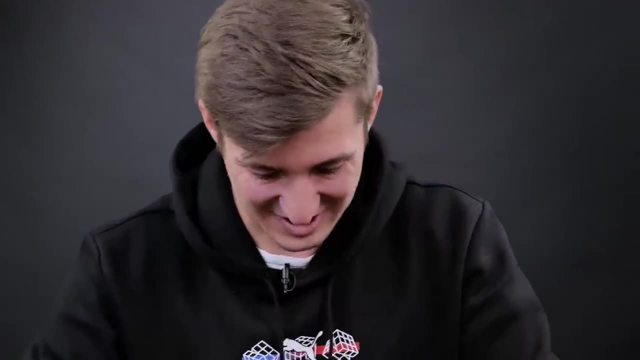 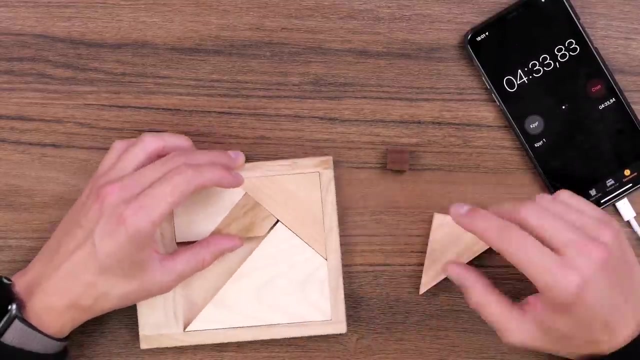 It can be like this: Damnurgh, It's unreal. Okay, okay, okay, Okay, you don't need it. Alright, no problem, Let us go, let us try…. As you can see, we have free space here. It means that we are doing something wrong. And what if we swap this? 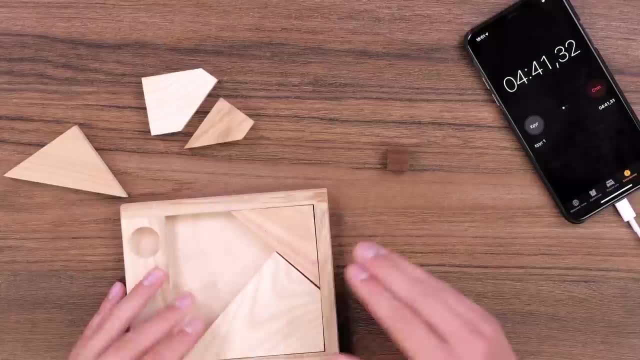 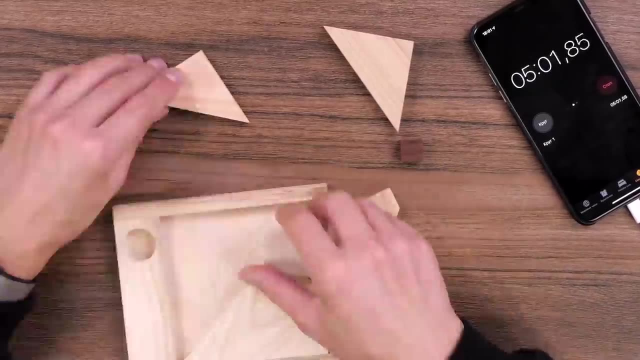 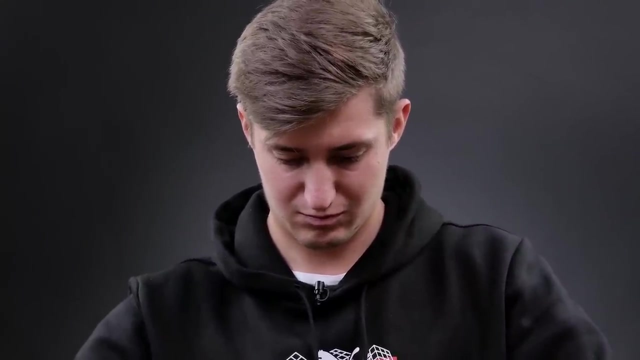 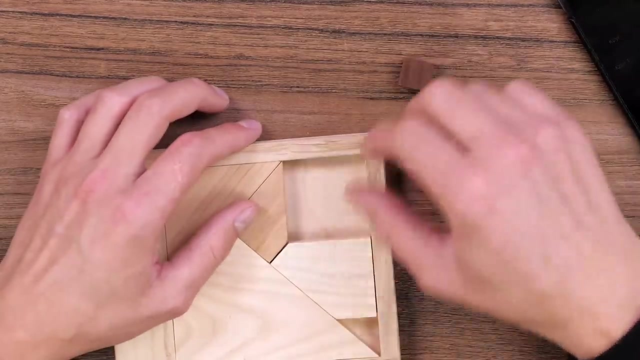 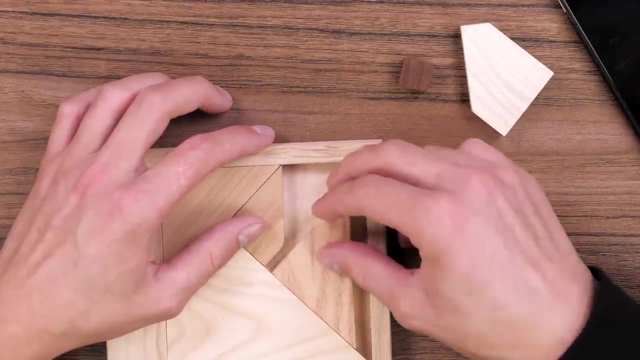 triangle, for that smaller one and then go further. Let's turn over this detail. We still have a lot of free space here Now. we have a lot of free space for the square and a few space for the triangle. Unreal, It looks so uneasy. 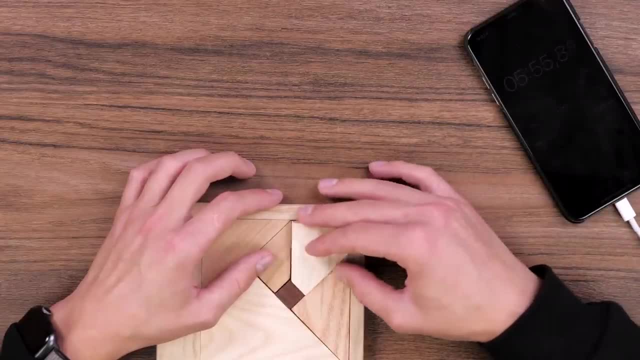 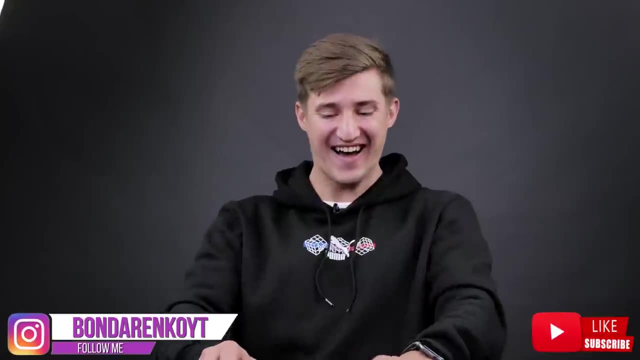 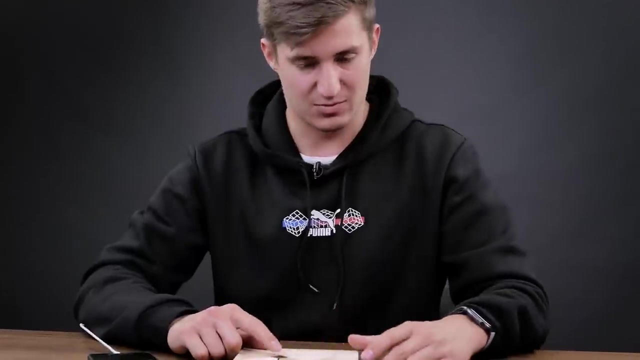 I think we're getting closer. Yes, Yes, Only 5 minutes- Awesome, Damn Ha-ha. And there is much free space left here. I can't believe that it's for real. This square requires much free space. It is large. 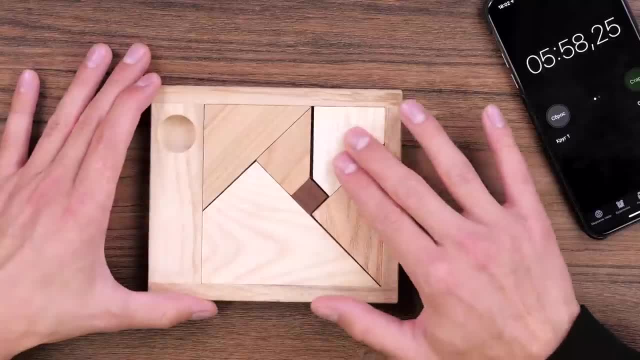 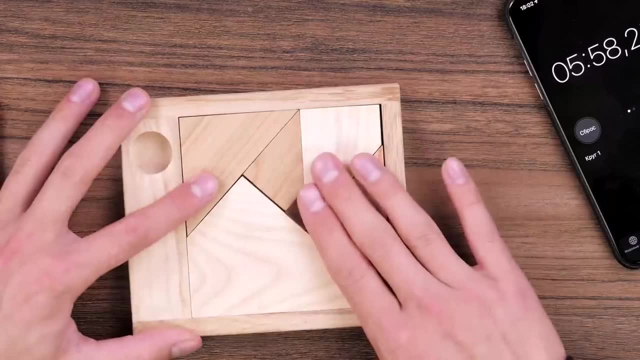 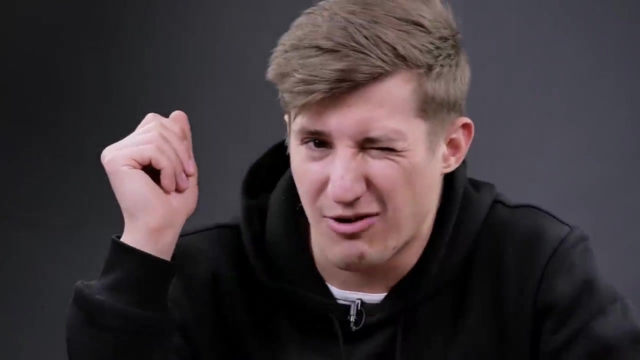 With one and a half centimeters, But we still have much free space between other details, Though at the beginning the frame was filled almost the same, It's so cool. It means that, firstly, geometry is a very interesting thing And, secondly, nothing is impossible. 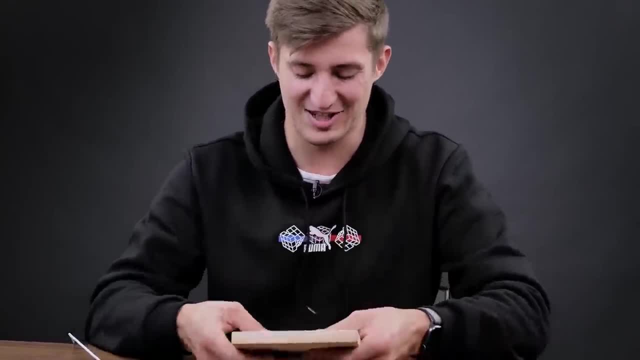 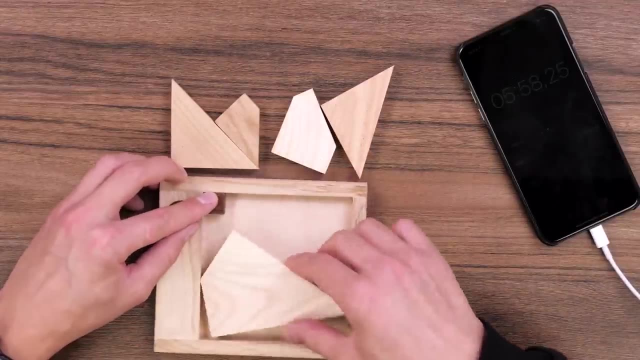 Let's find another solution. I think you want to find it. I hope that there are many solution variants. And of course, there are many solutions And the problem is that maybe I won't remember how I solved the puzzle the first time. 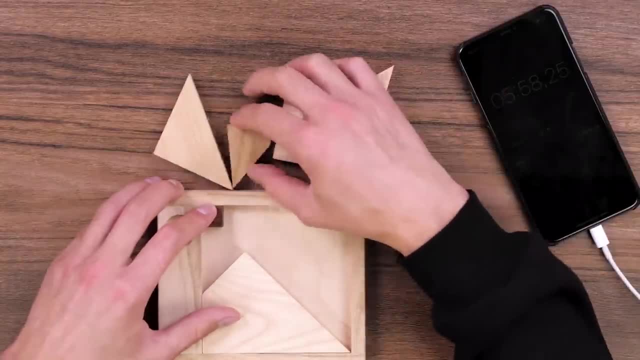 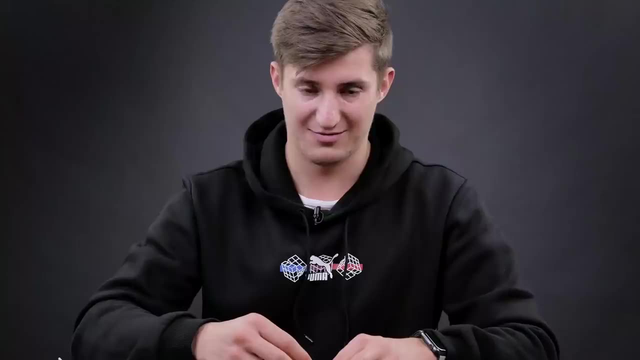 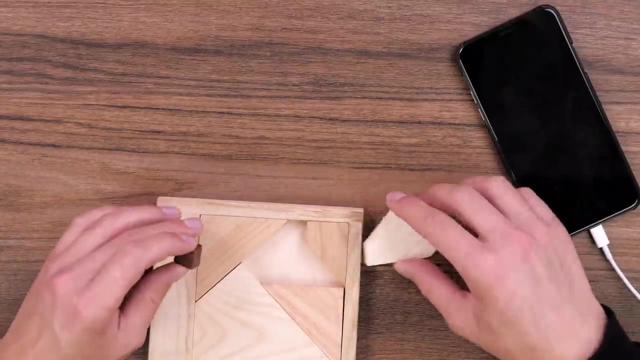 And I can solve it the same way twice. So let me know in the comments that I'm awesome, Isn't it? It seems to me that I'm repeating the same variant I did before. I'm sorry, Bye, Bye, Bye. 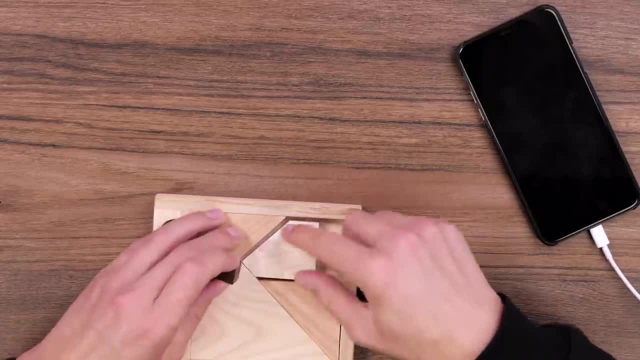 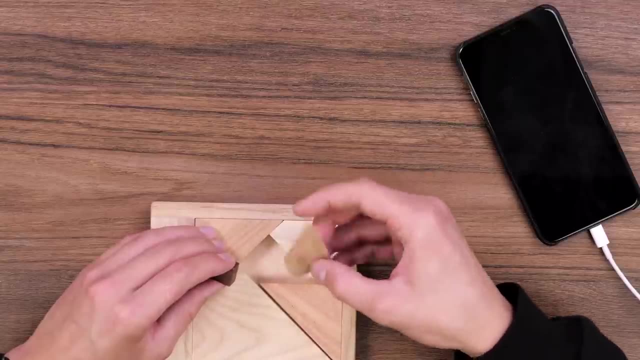 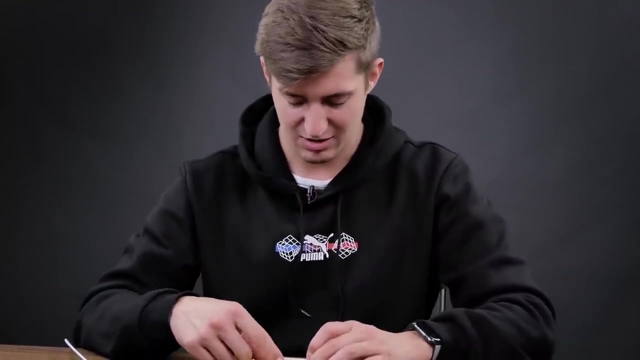 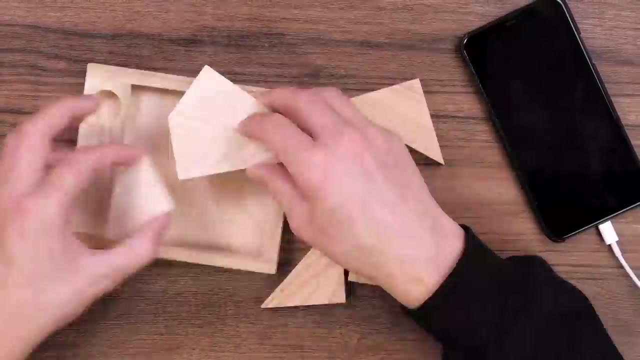 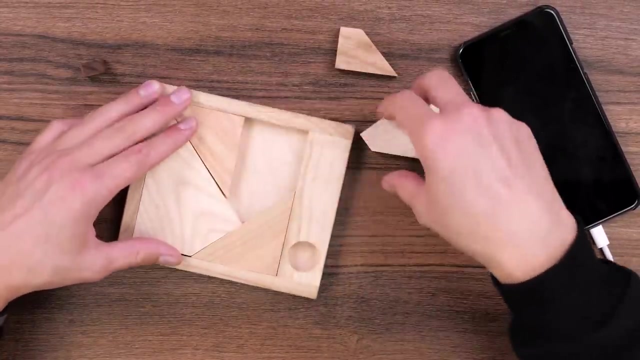 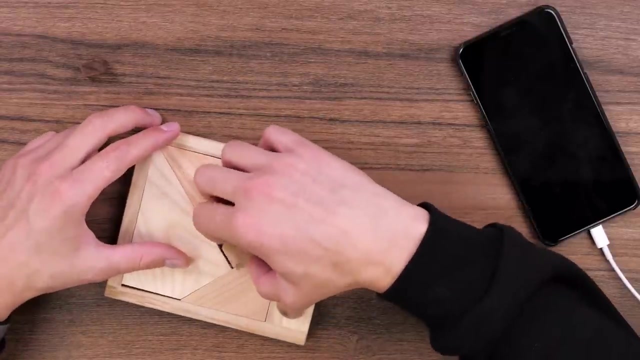 Bye, I'm doing something wrong. This is a departure position. I have already picked up several of them up. Well, Cool, I like it. And now I don't know how it should look like this, But we just need to swap the triangles. 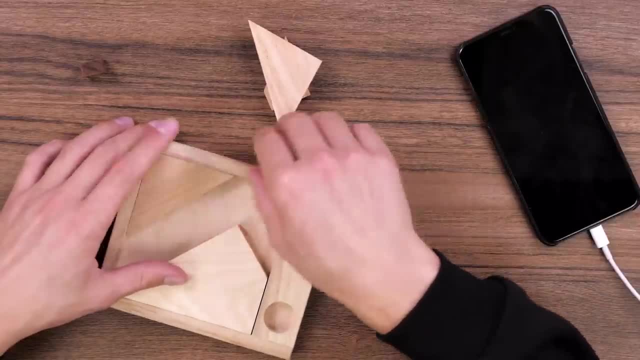 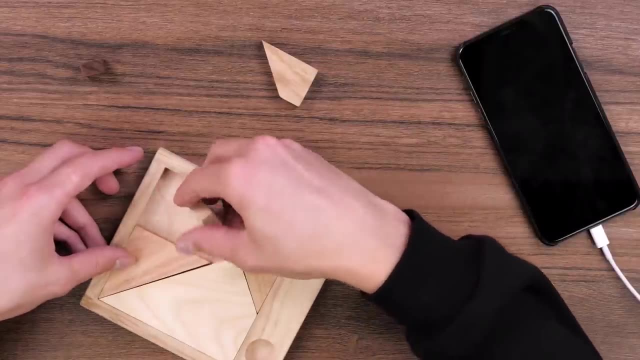 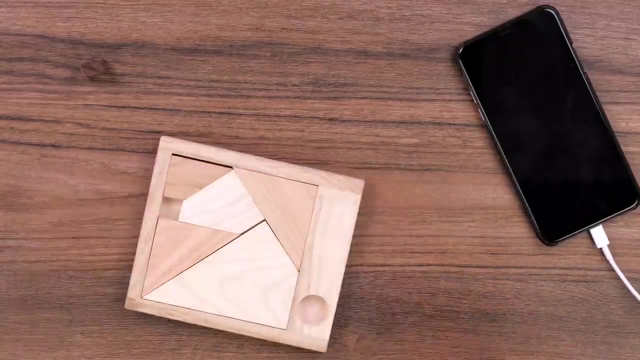 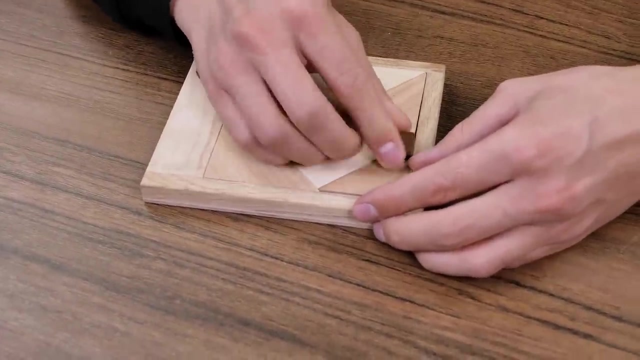 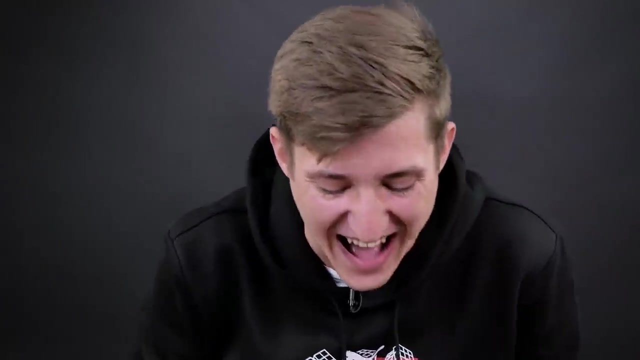 How it was like this, no, this one. I Have found a second solution. Guys, you won't believe me, but I have already shot the ending for this video Without finding the second solution, and I found it right now. Damn, that was cool. Let it be a bonus.